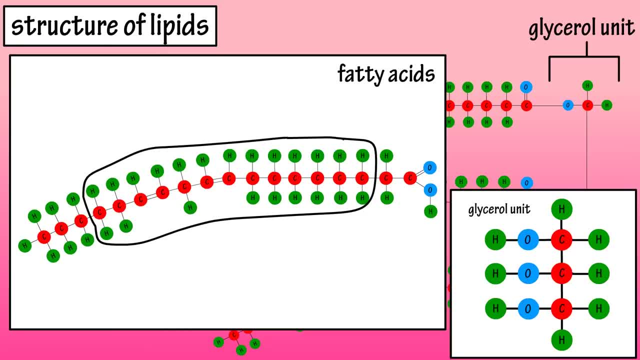 Atom. Fatty acids are made up of long chains of carbon atoms and hydrogen atoms, with an end carbon atom bonded to a hydroxyl OH group and a double bond to an oxygen atom. Some carbon atoms are linked by single bonds and others by double bonds. These bonds determine which type of fatty 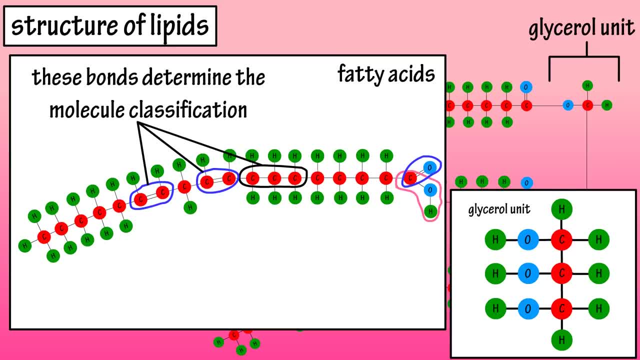 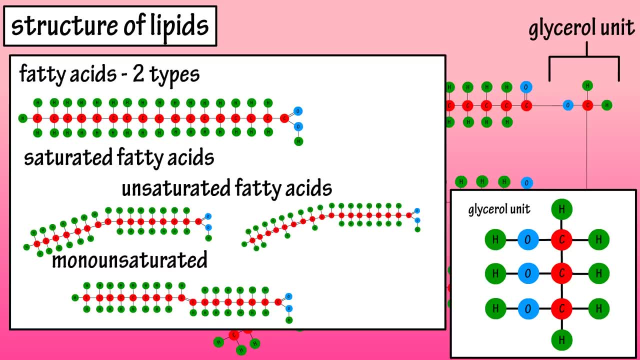 acid. the molecule is classified as There are two types of fatty acids: saturated fatty acids and unsaturated fatty acids, which include monounsaturated fatty acids, polyunsaturated fatty acids and trans fatty acids. We will cover fatty acid molecules in depth in a separate video. In the formation of a triglyceride, the fatty acids bond with the. 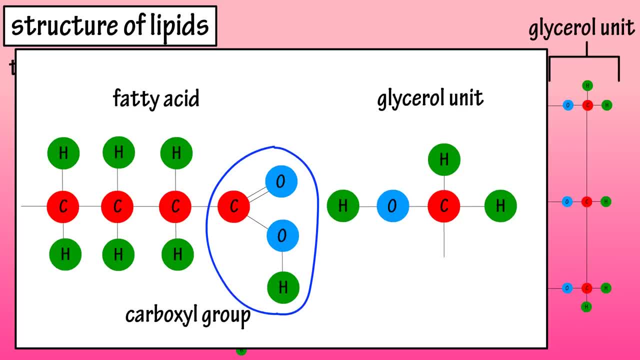 glycerol molecule. The three fatty acids attach their carboxyl groups, which are the carbon oxygen oxygen hydrogen group at the end of the molecule, to the hydroxyl OH groups of the glycerol molecule. As this process takes place, three molecules of water. 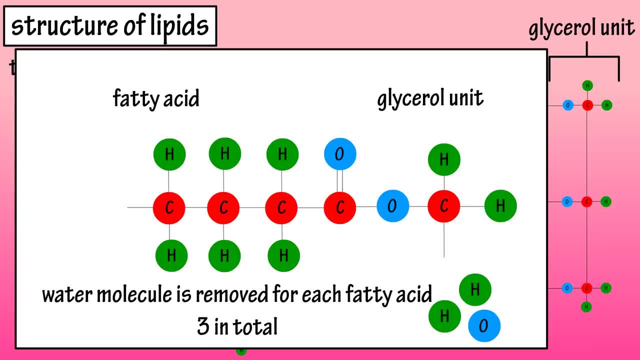 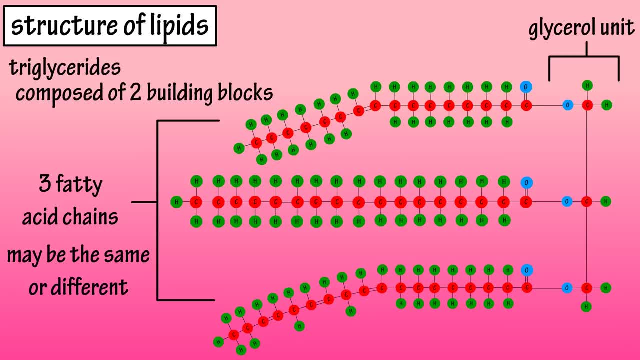 are removed, which is a dehydration synthesis reaction. Some triglycerides contain three molecules of the same type of fatty acid, and others may have three different types of fatty acids. Triglycerides are found in many food items, such as vegetable oils, coconut oil. 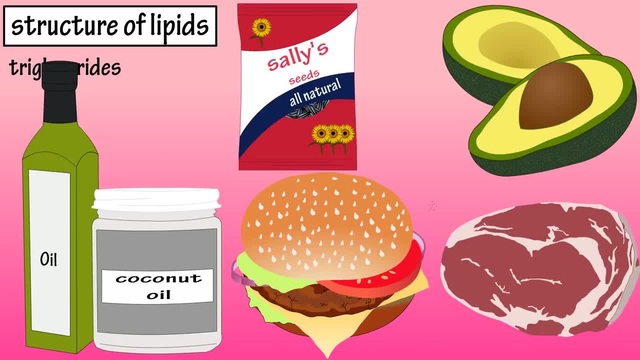 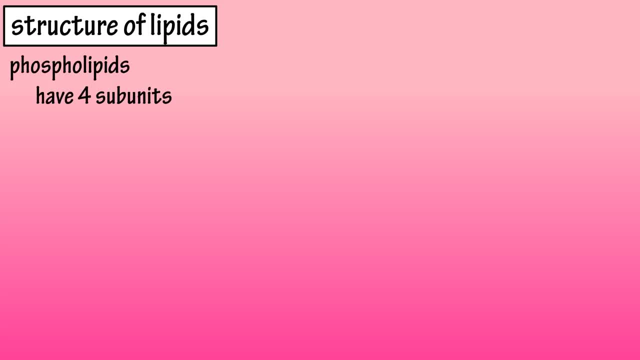 beef, fast foods, avocados and many different seeds. Phospholipids are similar in structure to triglycerides in that they have four subunits. They are composed of a glycerol unit, two fatty acids and a monounsaturated fatty acid. 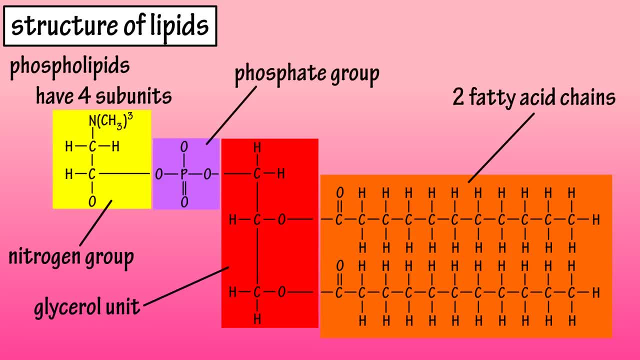 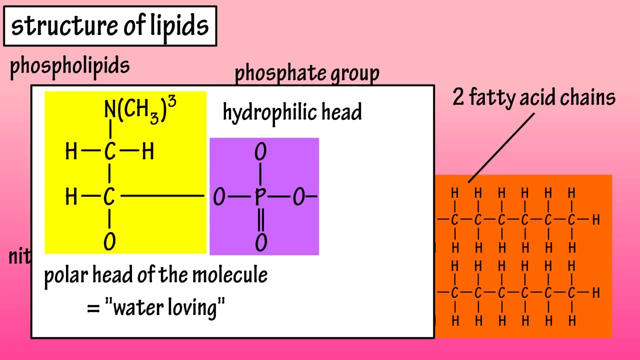 A phosphate group and a nitrogen-containing group. The phosphate and nitrogen group extend in the opposite direction of the fatty acids. This end, or the head, of the molecule is actually polar, so it's water-soluble. Hydrophilic, meaning water-loving, is the term often used. 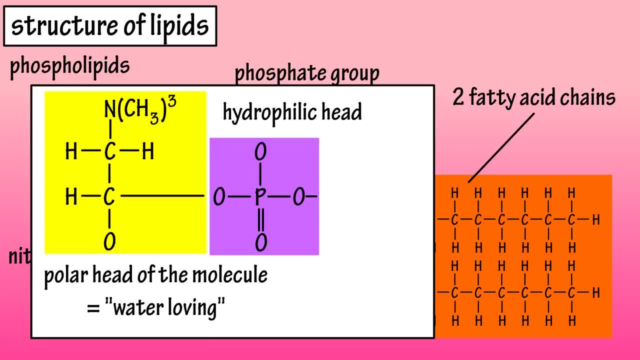 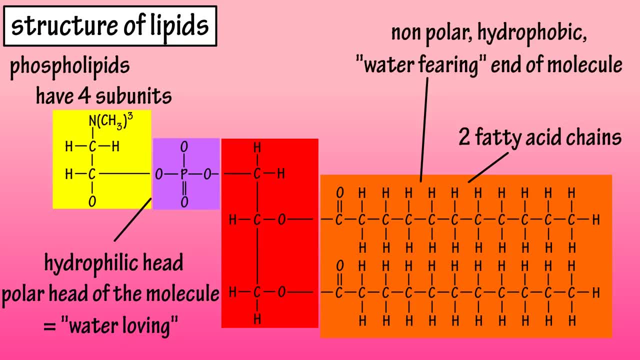 to describe the head portion of a phospholipid molecule. The fatty acids end is non-polar, so it's called hydrophobic, which means water-fearing. This property, having a hydrophilic and a hydrophobic region, allow this molecule to. 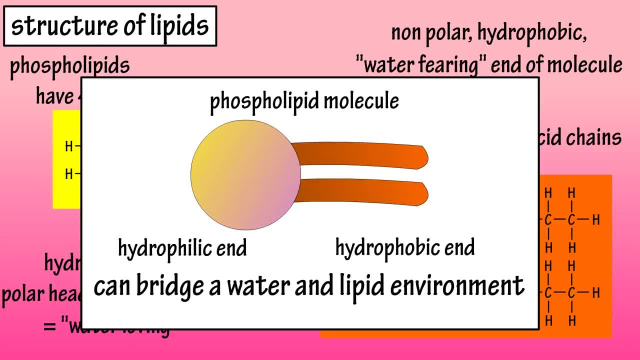 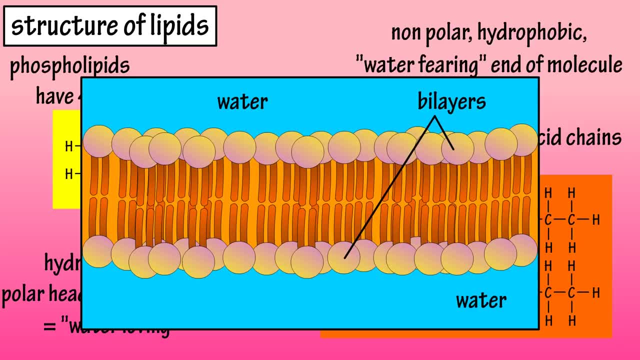 join or bridge a water environment and a lipid environment. So in water these molecules will form bilayers, with the fatty acid tails facing each other and the heads facing outwards, as you can see here. Phospholipids are the main component of cell membranes. Steroids, which are often